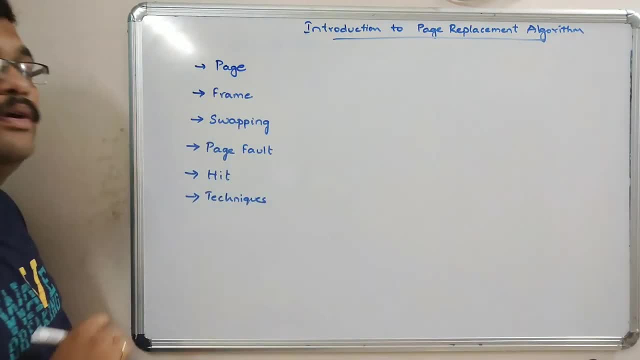 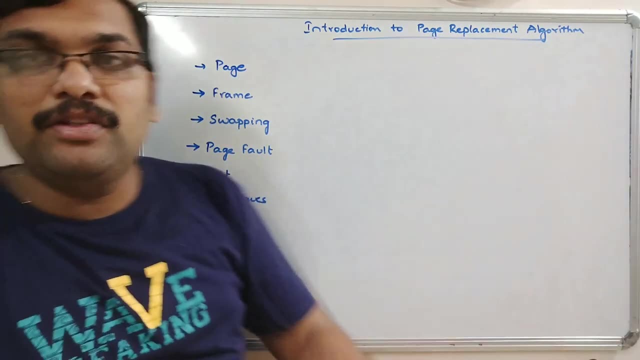 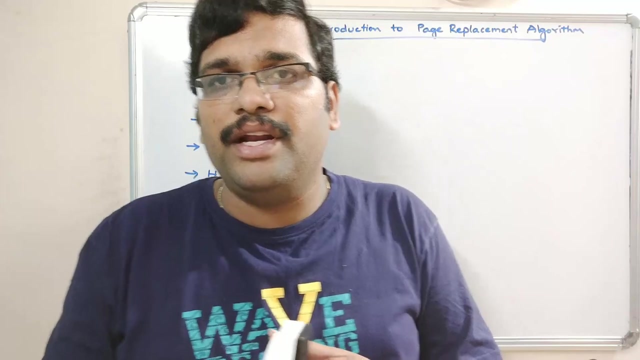 used right. so page frame swapping, page font hit and techniques now coming to this page replacement algorithm. we know that. so the processor will load the process which is going to be executed into the main memory from the secondary memory. so we know that all the files and all the 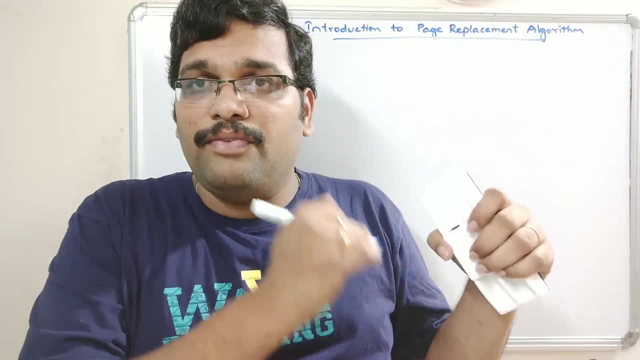 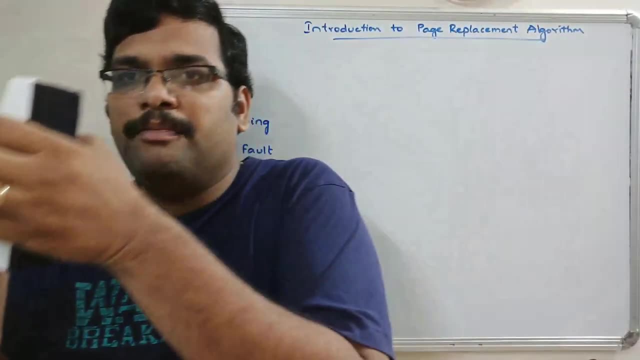 processes will be stored in the secondary memory. so whenever we are executing the process or a file, whenever we are loading the file, that file or that process will be loaded into the main memory and then it will be executed. so for execution of the process it should be loaded from the secondary memory. 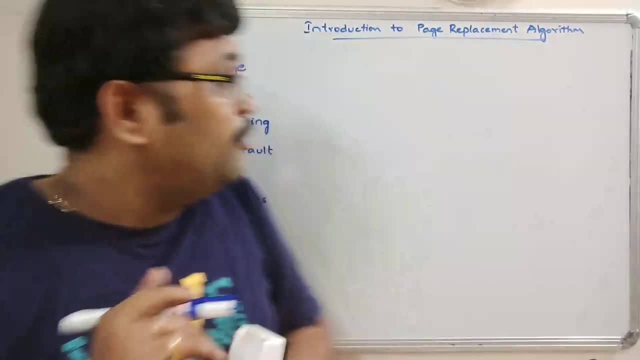 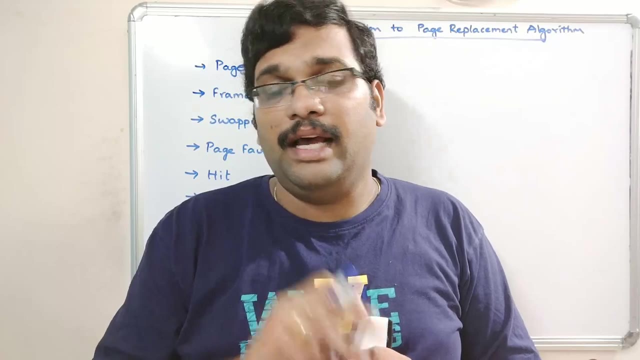 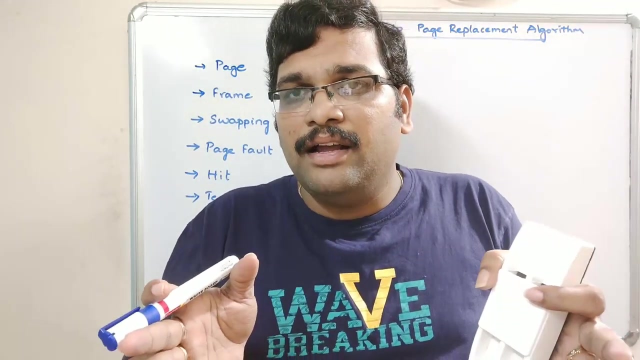 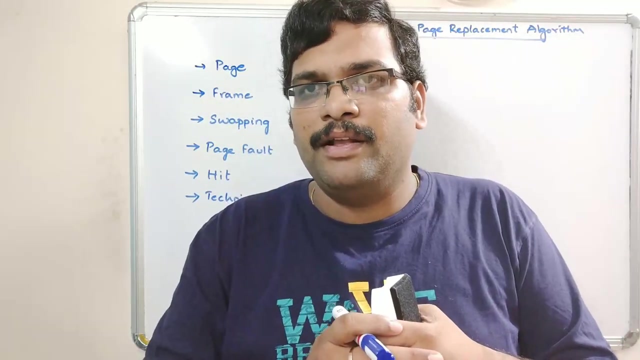 to main memory. that is the important concept right now. the question is: is it required to load the complete process into the main memory? the answer is no, so here the process will be divided into different parts, and each part will be loaded from the secondary memory to the main memory whenever it is required, so that 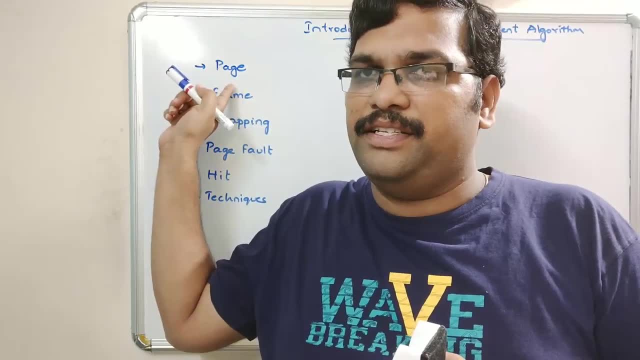 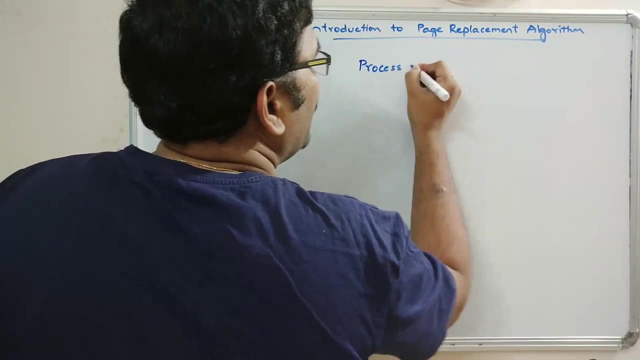 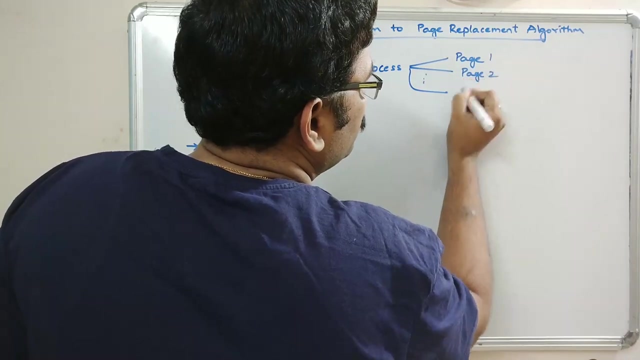 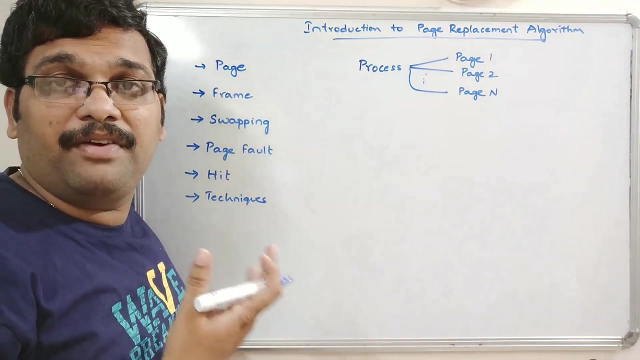 each part of the process is called page, So process will be having pages: page 1,, page 2,, page n. So there will be page number right. So a process can be divided into number of pages n number of pages. Now, this is about the page. It is a part of a process. 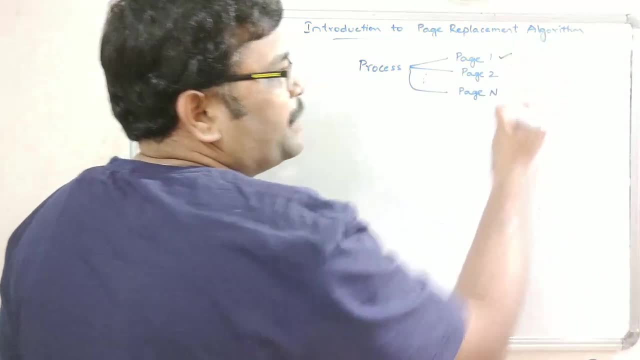 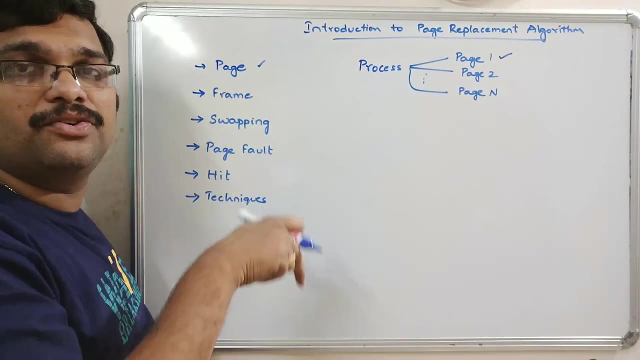 It is a part of a process. So if we want to execute this page 1, first the page 1 should be loaded from the secondary memory to main memory and then only it will be get executed by the processor. Now, coming to this frame, Similar to the process, the main memory is: 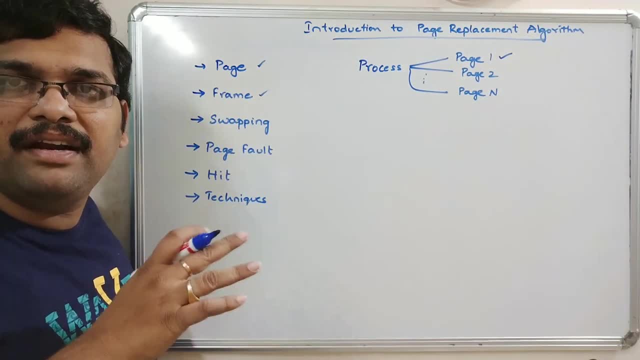 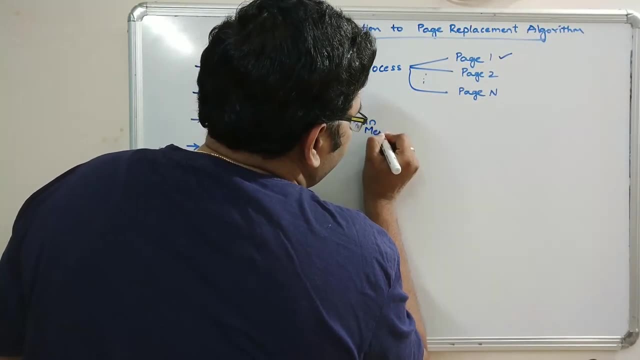 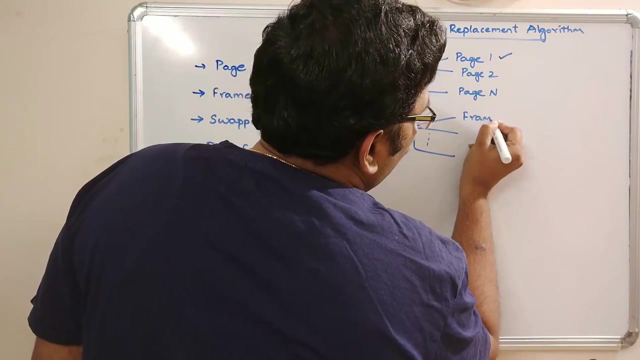 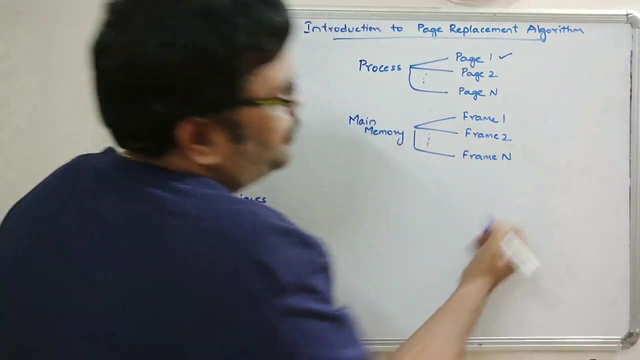 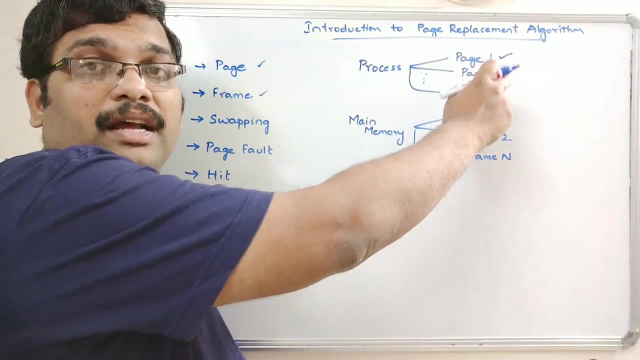 also finite and the main memory is also divided into different frames, See main memory. so frame 1, frame 2, frame n. right Now, if page 1 is to be get executed, the page 1 should be loaded from the secondary memory to main memory in one amount. 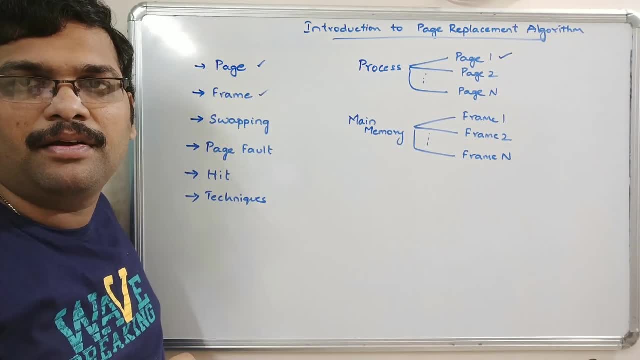 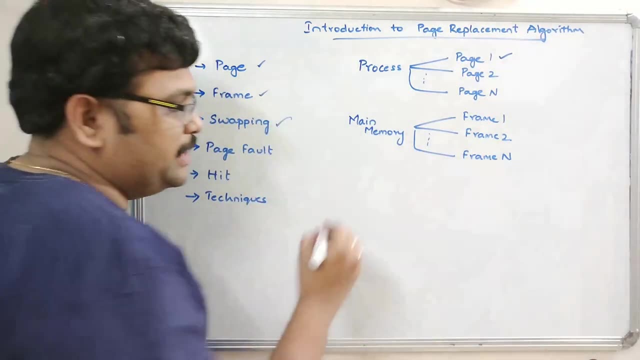 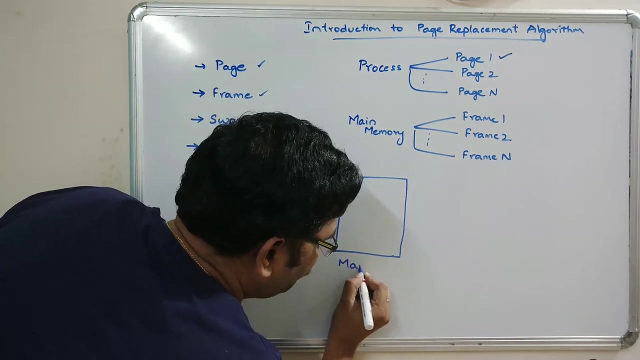 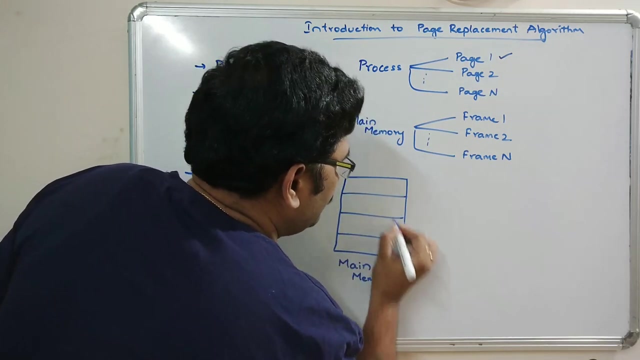 So the main memory is of these frames which is available, right? So this is a frame. Frame is a part of main memory Swapping. see, this is a main memory. See, this is a frame 1, frame 2, frame 3, frame 4, frame 5, frame 6, frame 7, frame 8, frame 9, frame. 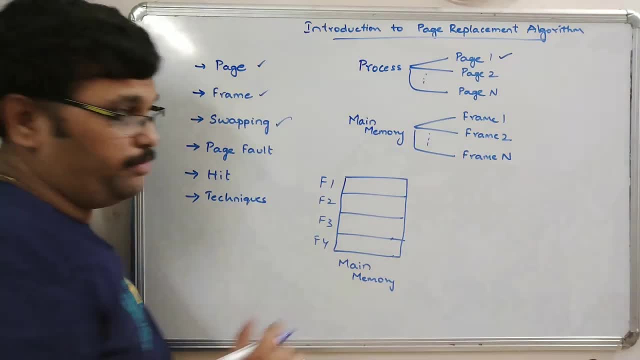 10, frame 11, frame 12, frame 13, frame 14,, frame 15.. Let us see, this is a frame 1, frame, Frame four. so memory is divided into four threads. Similarly, We are having some process. 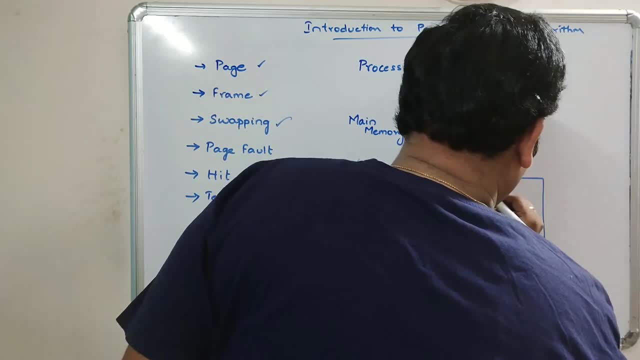 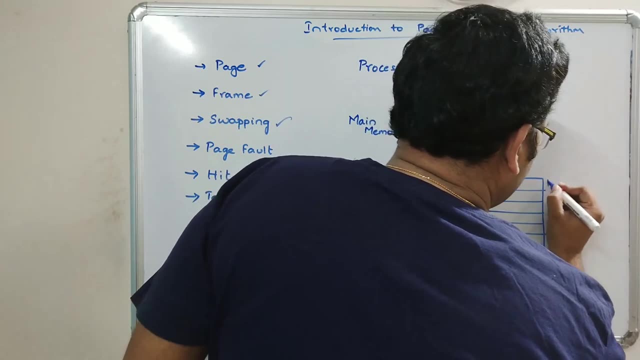 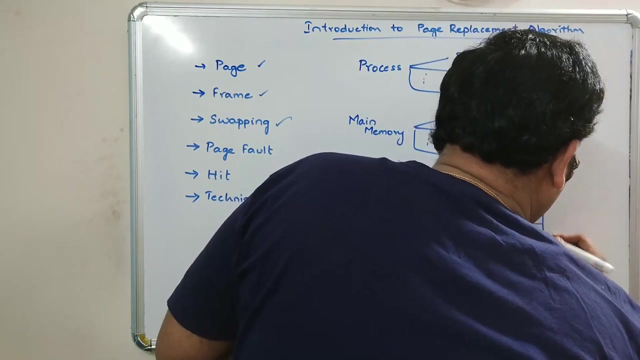 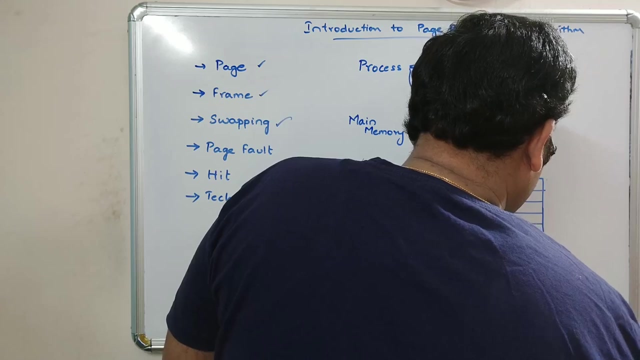 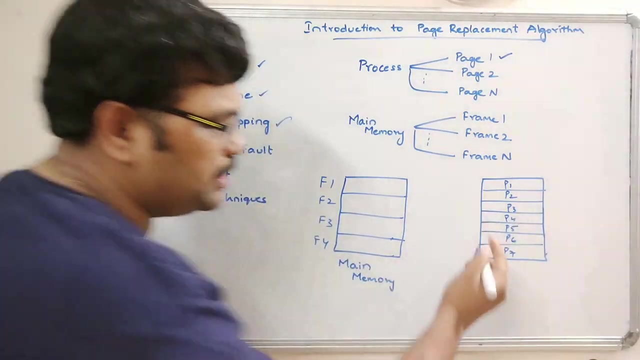 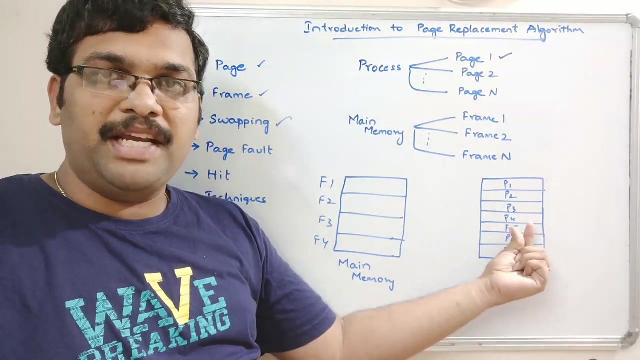 P1, P2, P3, P4, P5, P6, P7. So there are here. P1 is nothing but a page one, Page two, page three. So this is a process, right? If you want to execute this process first, we have to load these pages into these frames. 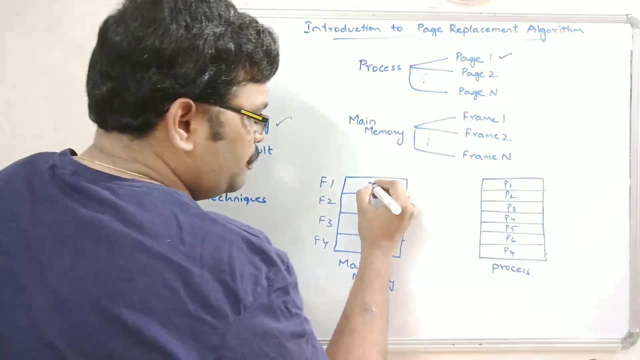 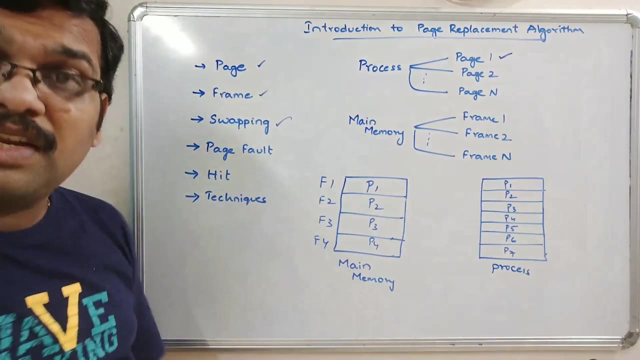 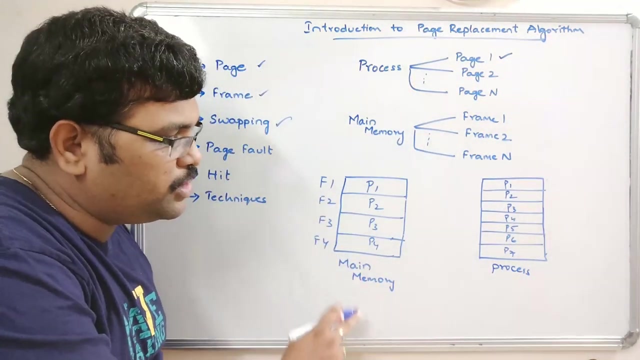 So see, we are executing this one. So page one is here. next page two is here. page three is here. page four is here Now the processor want to execute the page five. right Now, the process. I mean the processor wants to execute page. 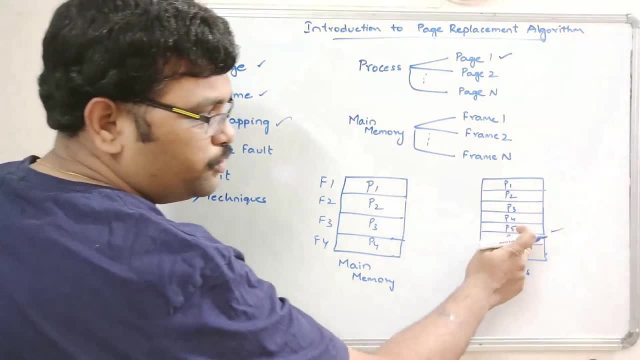 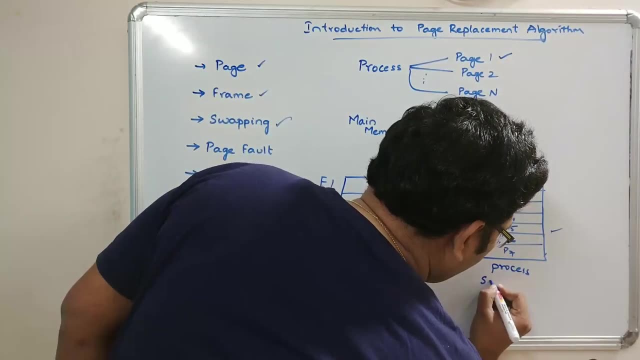 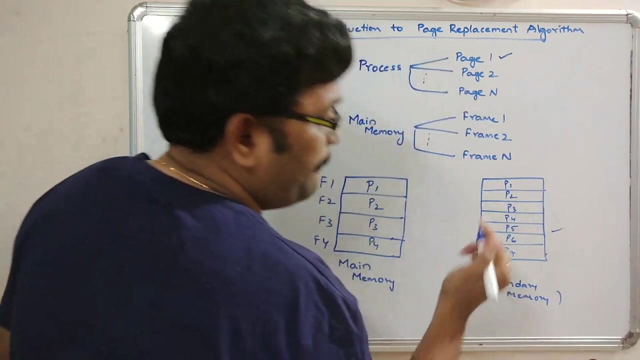 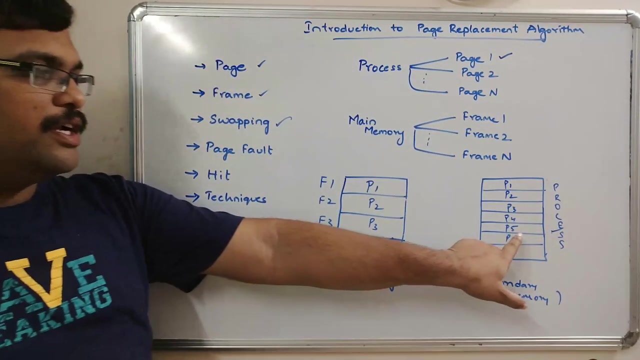 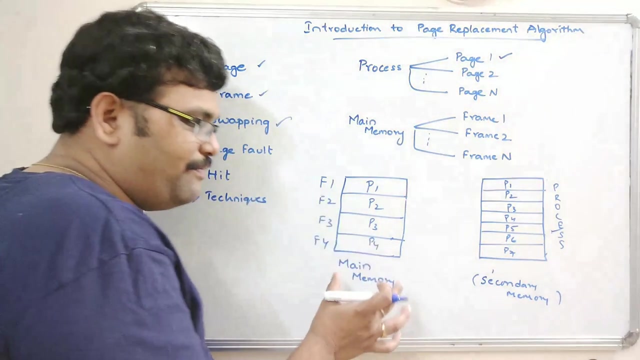 five. Now this page five should be loaded from the secondary memory to main memory. So this is the secondary memory. This is the process. So we wanted, the processor wants- to load this P5, execute this P5. So first the processor will check for the main memory. 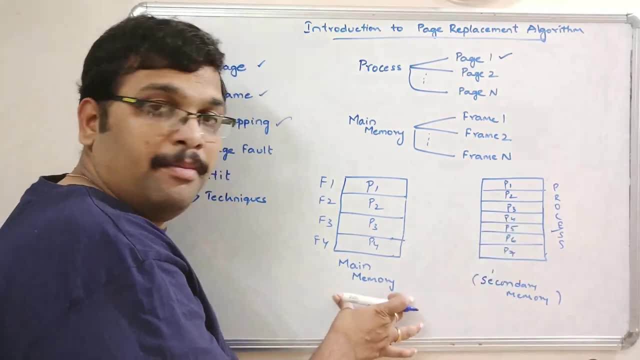 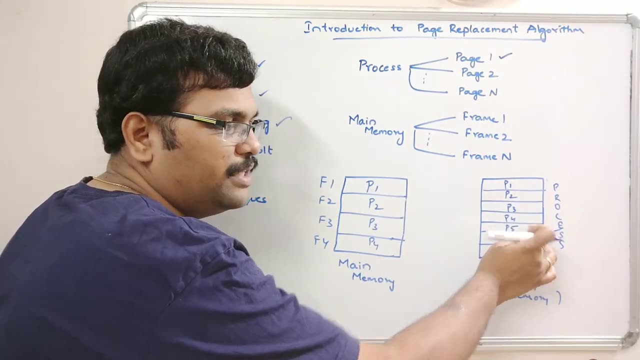 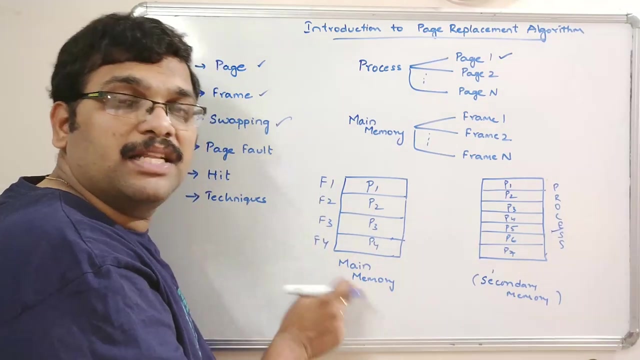 I mean check for this required page in the main memory. If it is not available, then it will load this required page from the secondary memory to main memory And before loading that, it will check for the availability of frames in the main memory. 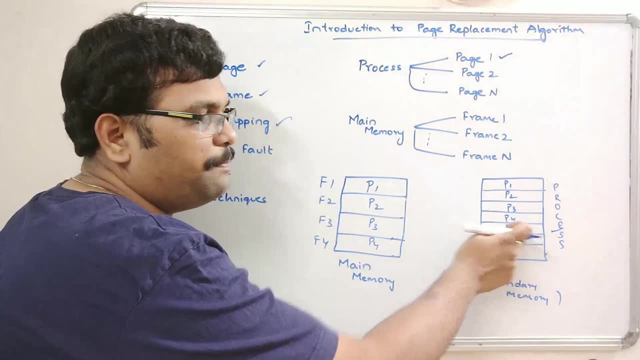 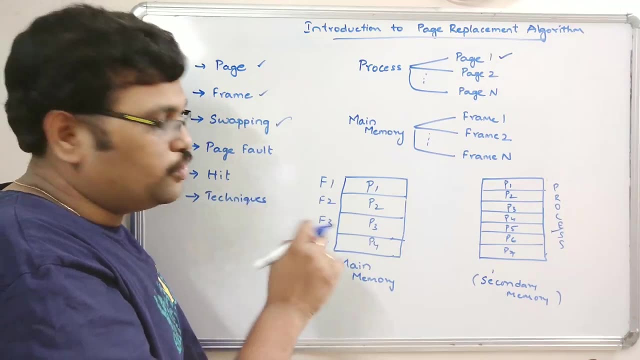 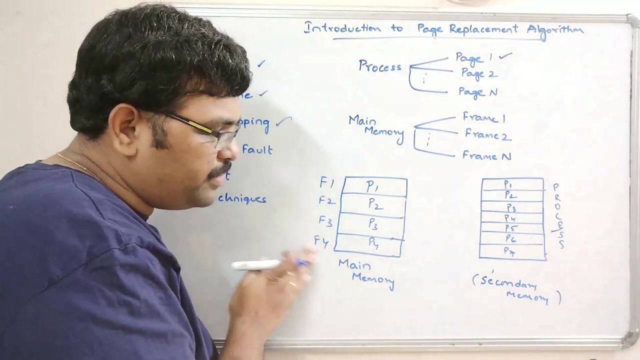 If it is available that directly, that required page will be loaded into the available frame, And if the frame is not available, what we have to do? So one page should be replaced with the required page. So in this example, so here, there are four frames in the main memory and already the four pages are filled in this frame. 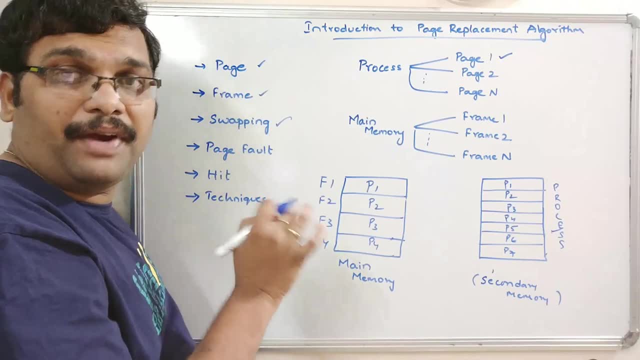 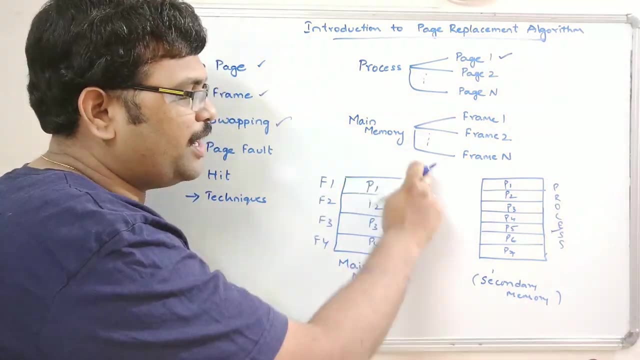 Now the processor wants to execute this P5, page five. So page five should be loaded from the secondary memory to main memory. But here no one frame is available. Not even one frame is not available. So we have to replace one page. 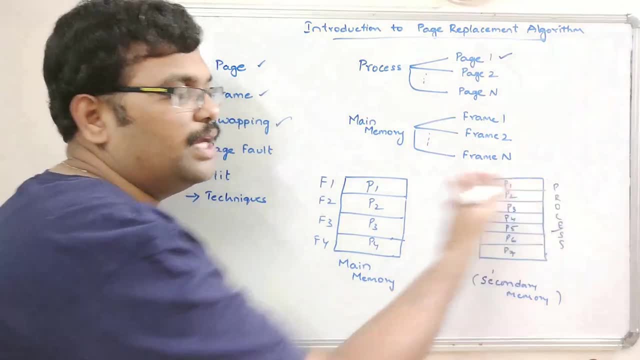 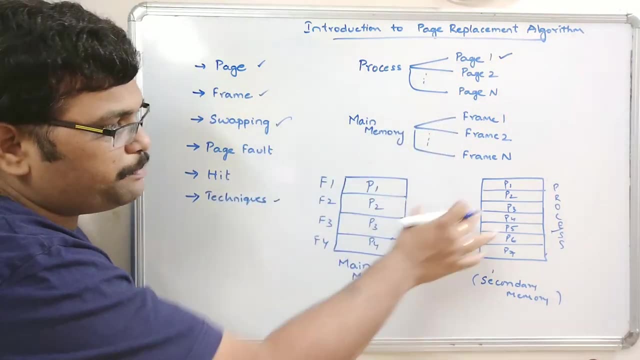 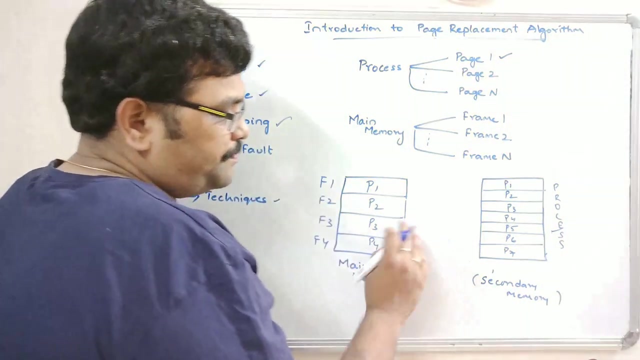 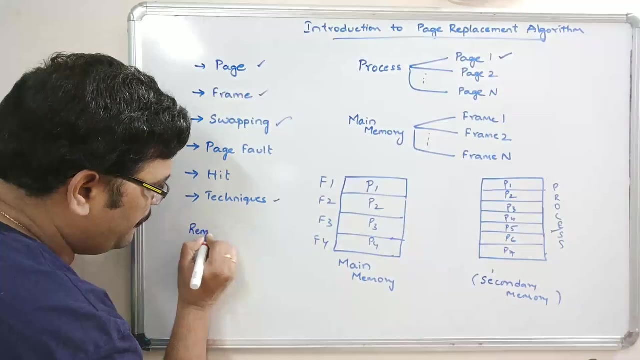 One page from the main memory with the required page. That is called the technique. So with the help of- sorry, this process, this process is called a swapping, Swapping, Okay. So here, replacing that means removing the page, Removing page from. 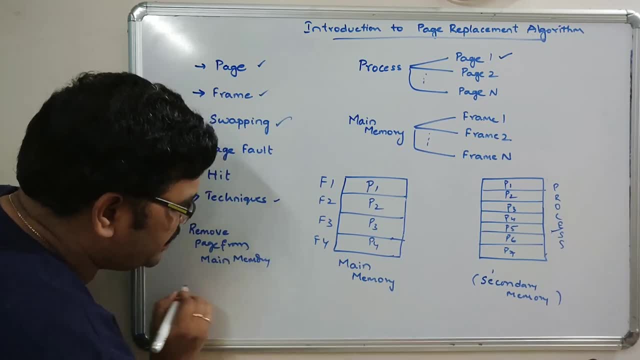 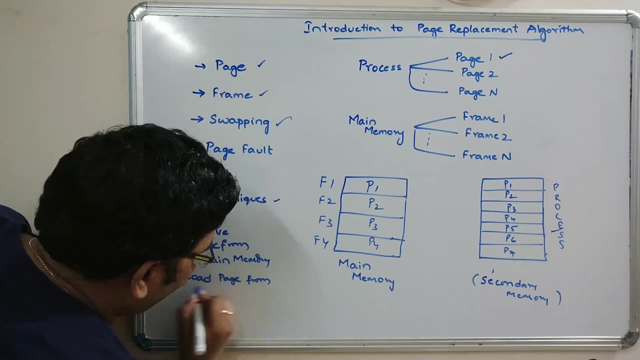 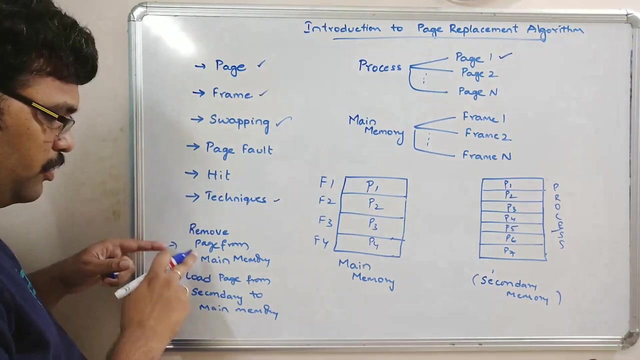 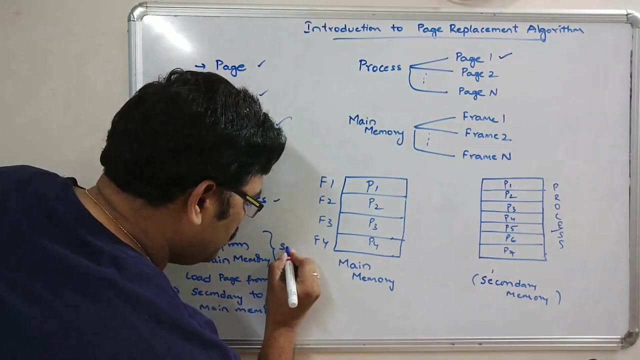 Main memory. That is one step Load Page From Secondary to Main memory. Okay, These are the two things must be happened. So before loading we have to check for the available frame. So this process is called Swap out. 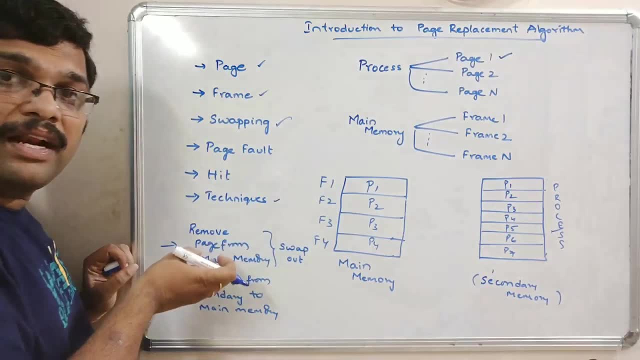 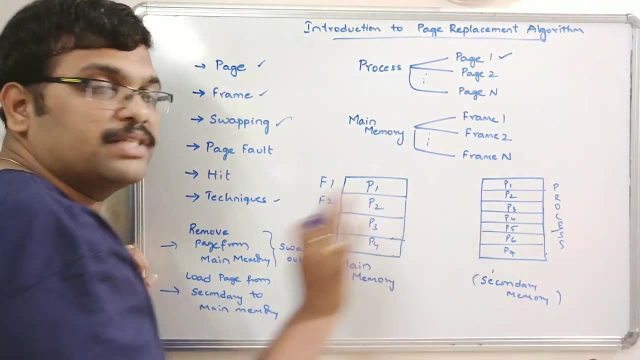 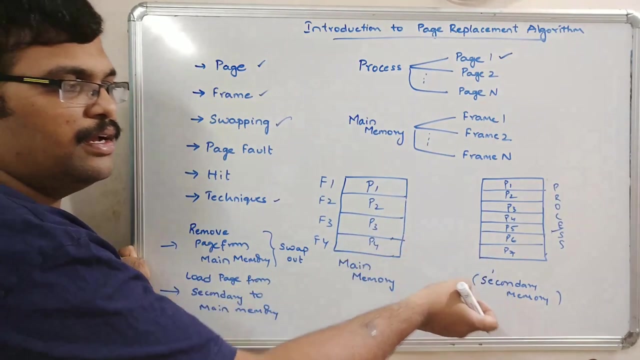 So because we are removing, that means we are removing the page- one page among the several- from the main memory to the secondary memory. So that is called swap out And immediately the required page will be loaded from the secondary memory to the available frame. 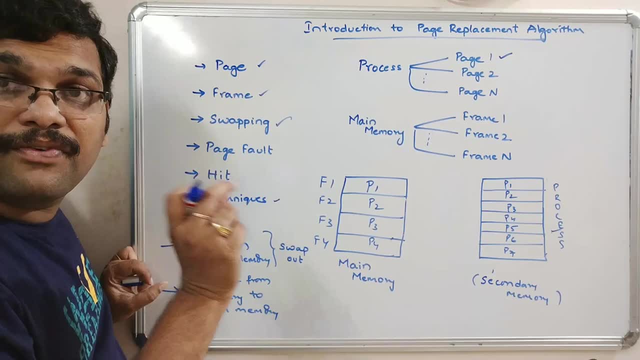 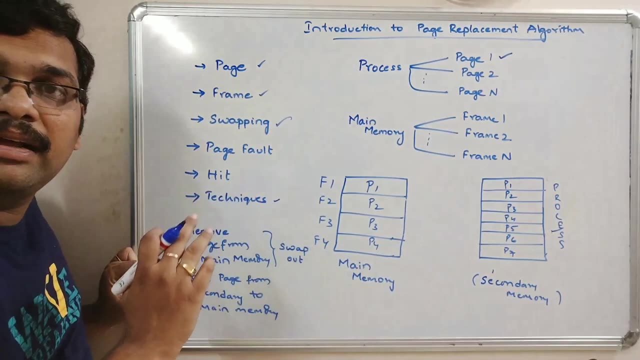 So if you remove the page from the main memory, That particular frame will be in a available state. So we have, we can load the required page from the secondary memory to the main memory. So available frame to the available frame. So this is called swap in. 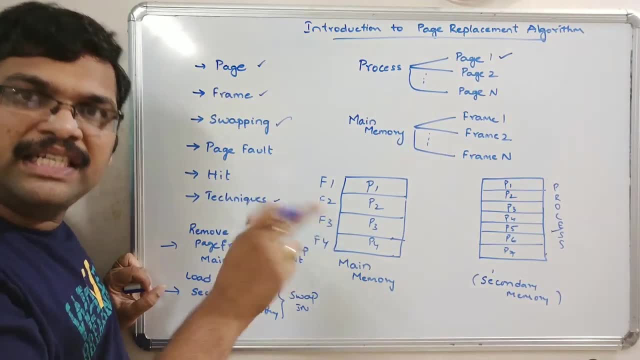 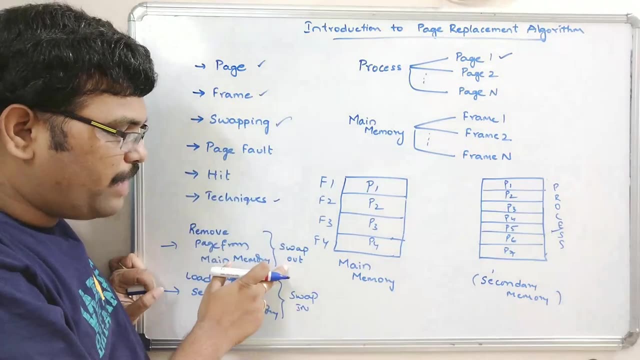 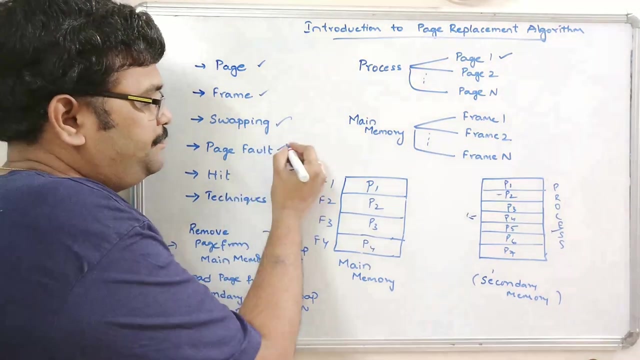 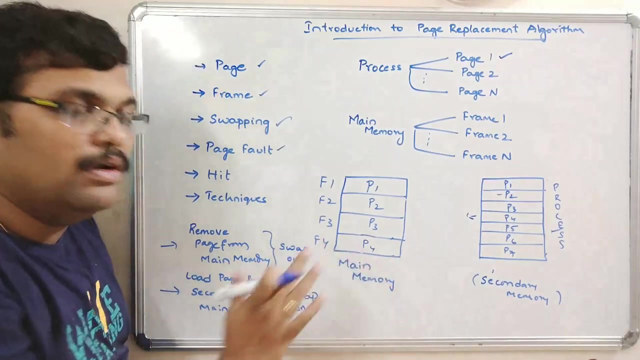 So finally, the process of switching the pages from secondary memory to load, secondary memory to main memory is called swapping, So that can be swap in or swap out Right Now. So page part. So page part means loading the page required page from the secondary memory to main memory. 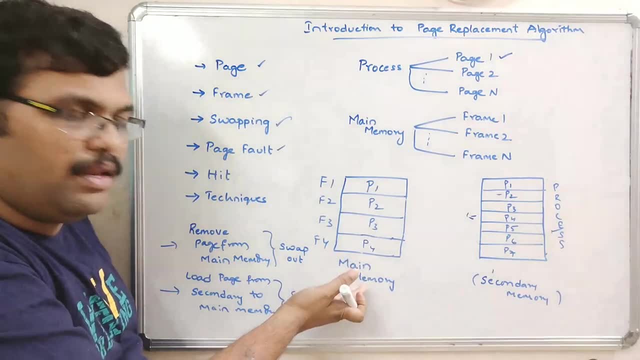 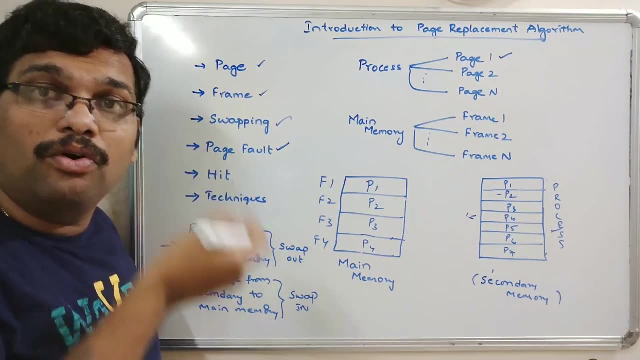 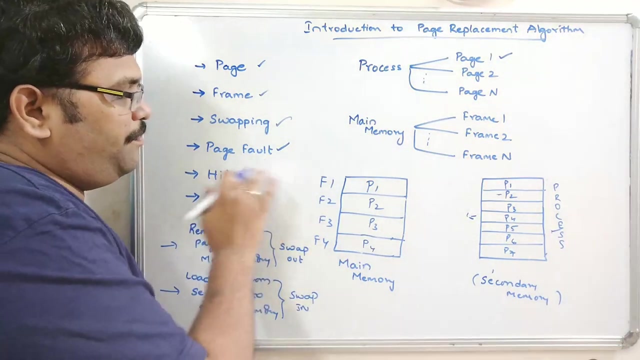 If the required page is not available in main memory, then that is called page part. So there is a page part. So we have to load the required page from the secondary memory to main memory, Right. So this is called a page part. 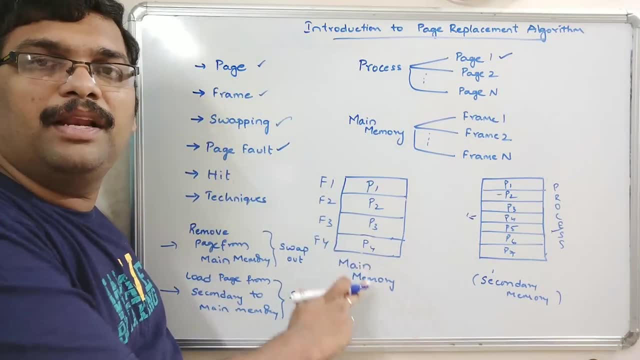 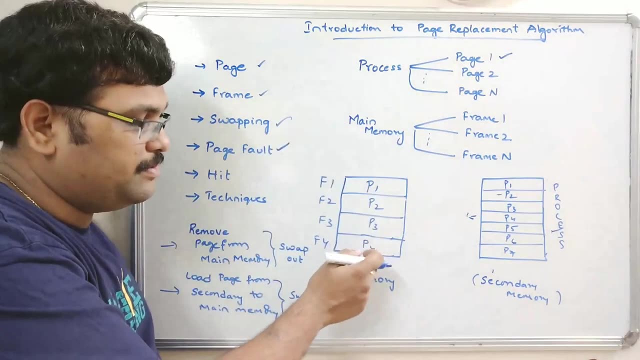 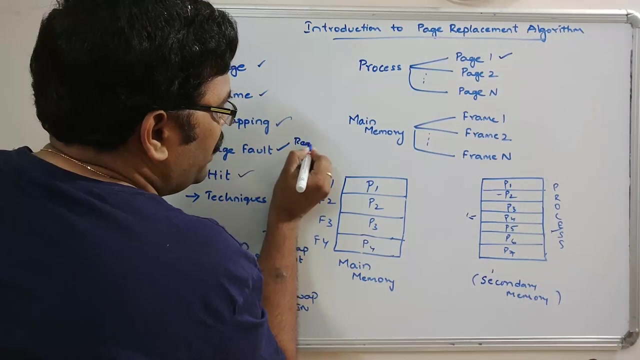 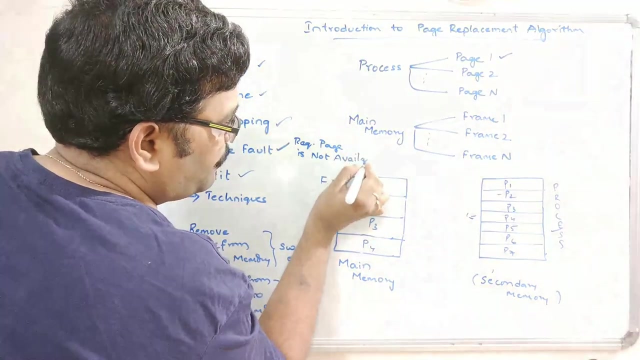 So that means the required page should not be available in the main memory. So that is called a page part. And if the required page is available in page part- I mean in main memory- that is called a key. So the required page is not available. 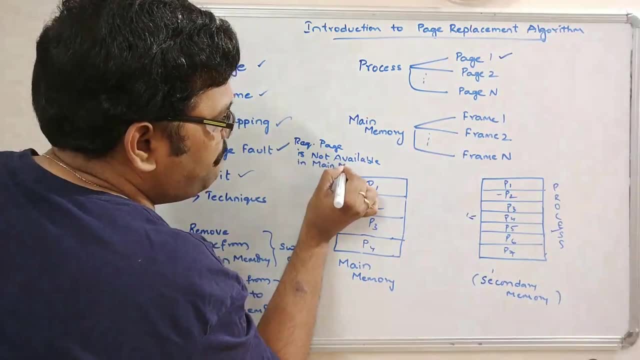 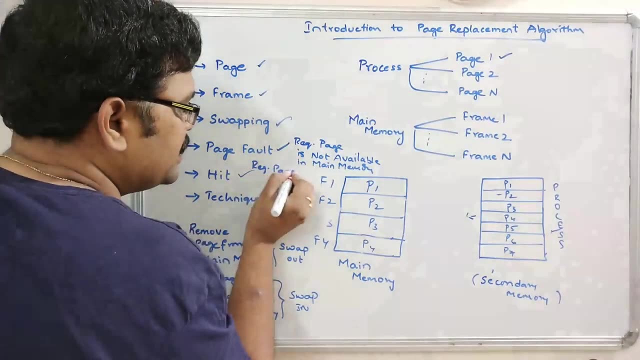 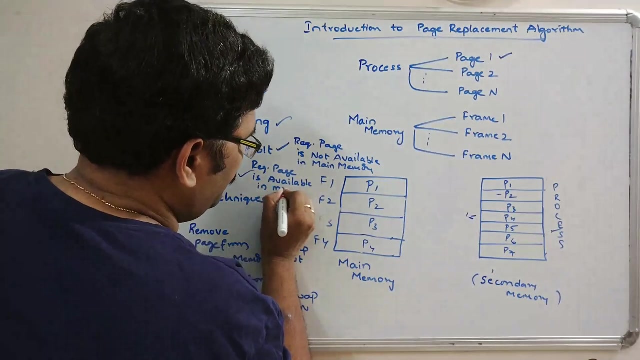 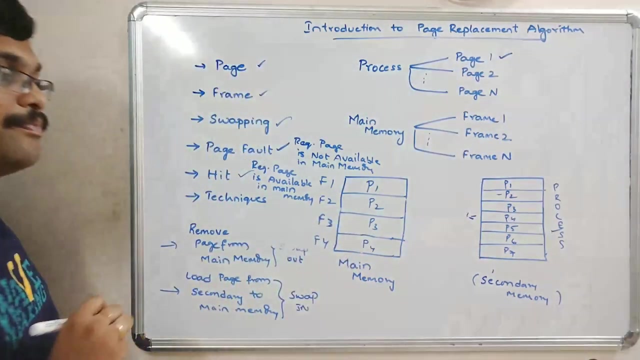 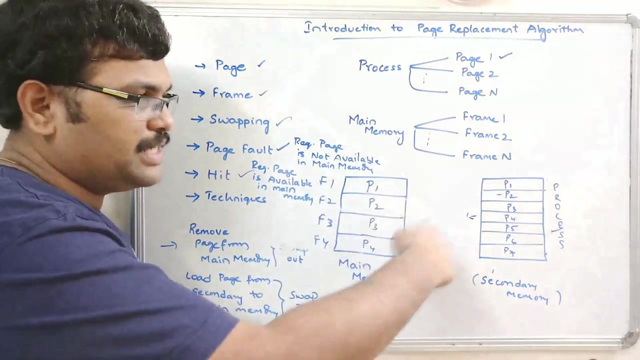 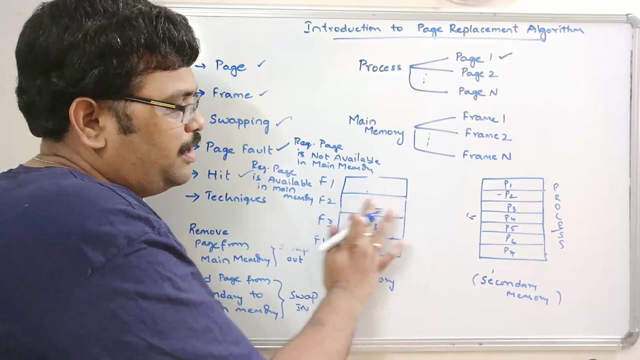 In main memory. It means the required page is available in main memory. Okay, Right See, For example. Now let us consider this example itself. So already all the frames are full, Right See? Okay, Let us take an empty frame. 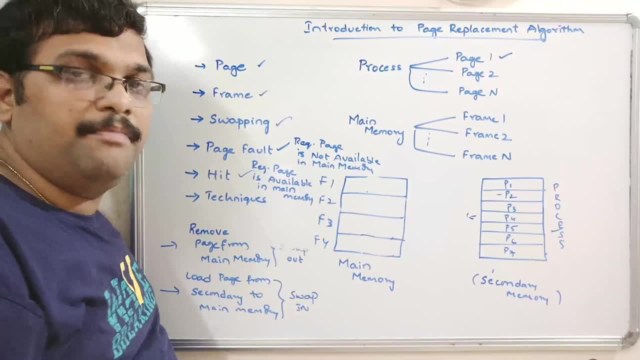 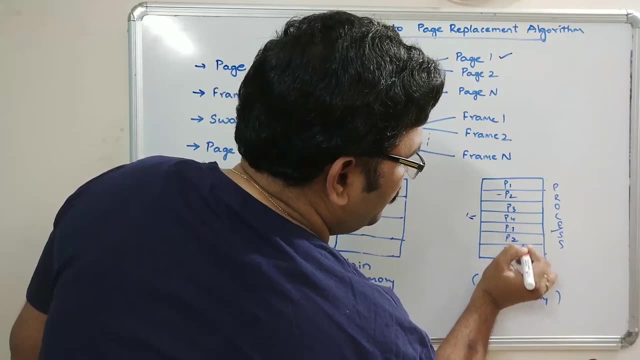 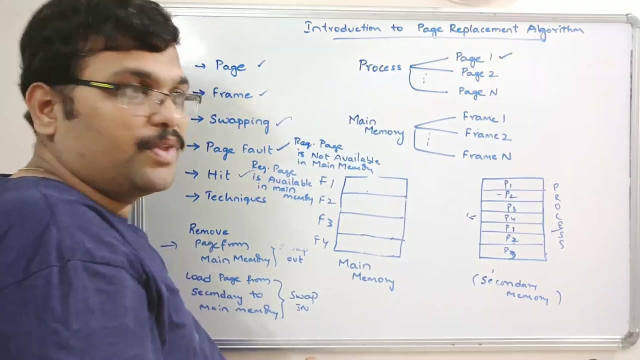 So let us start from the beginning. So the page sequence is same: The p1, p2, p3, p4, p5 and similarly, again sorry, p1, p2 and p3. The page sequence. The processor wants to execute the process in this way. 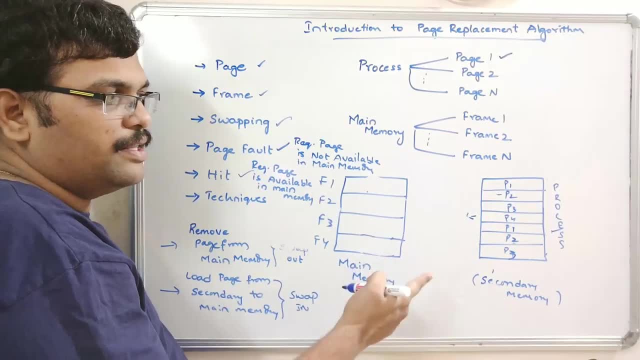 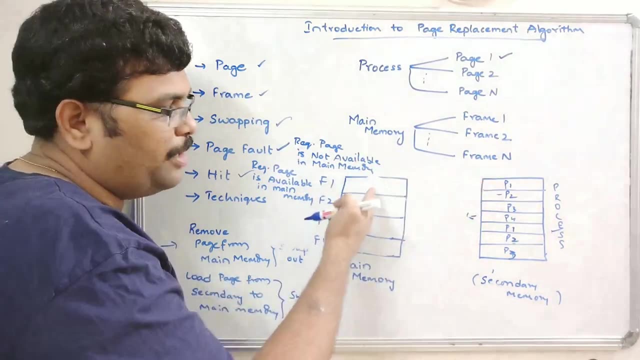 Okay, First of the p1.. First it will find the processor will find whether the page 1 is available in the frame. So all frames are empty. It is not available. So that means there is a page part. So p1 will be here. 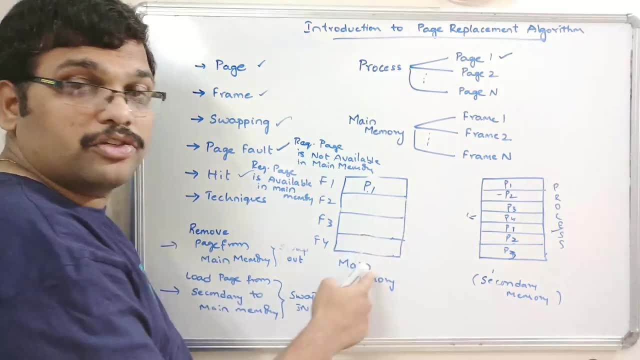 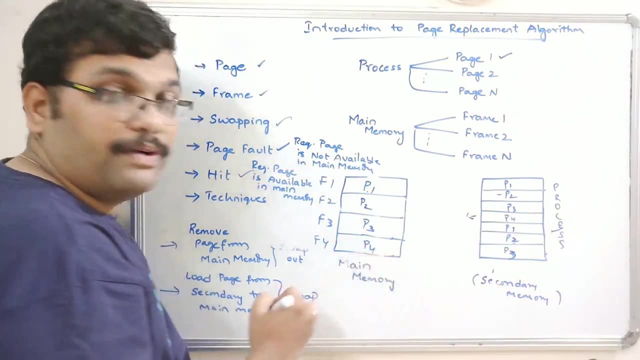 So there is one page part till now Coming to the p2.. p2 is also not available in main memory. Second page part: p3.. Third page part: p4.. Fourth page part, Again p1.. So p1 is already available in the main memory. 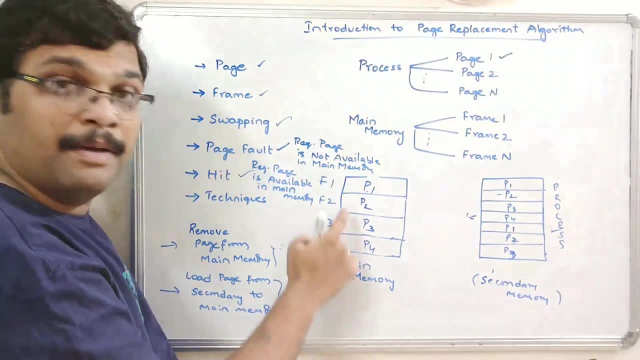 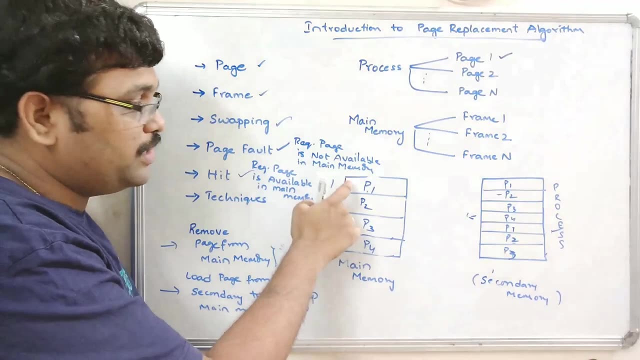 So p1 is already available in main memory. Okay, So we need not to swap any page. p1 is already available in this one. So there is no page fault. So there is one. hit Again: p2.. p2 is also available in main memory. 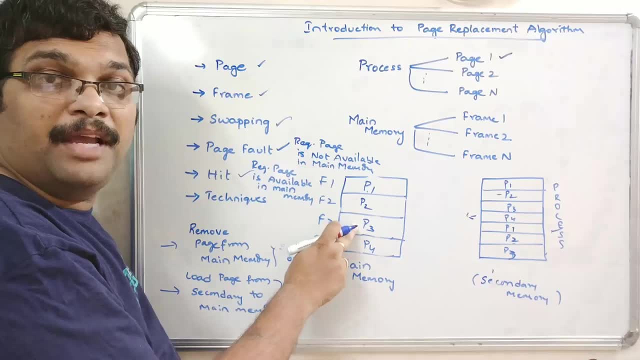 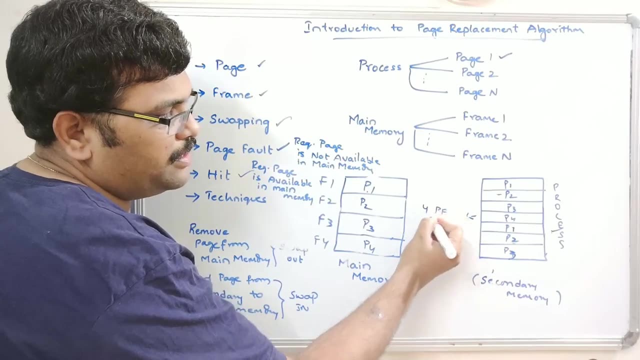 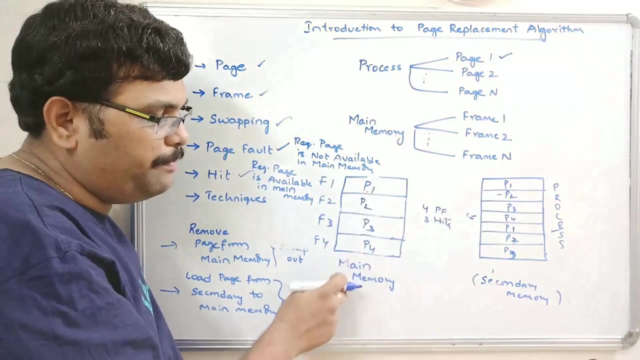 So second hit: p3.. p3 is also available in main memory, So third hit. So for executing this one, we are having four page faults and three hits. Hope you understood. So whether the required page is available in main memory, then we call it as a hit. 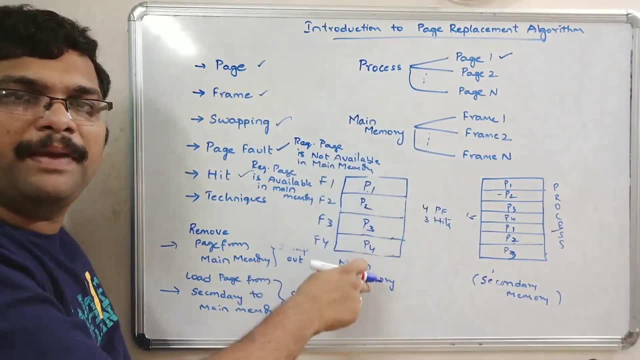 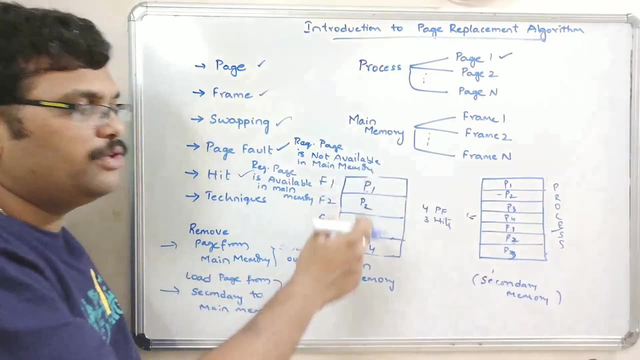 Whether the required page is not available in the main memory. that is called a page fault. So the next step of this page fault is we have to load the page into the memory. So for that we have to again check for the free slots of a memory. 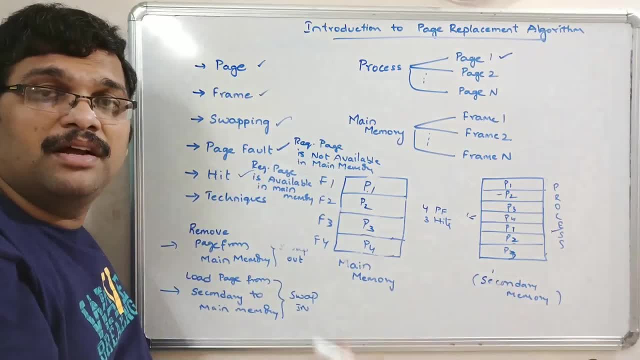 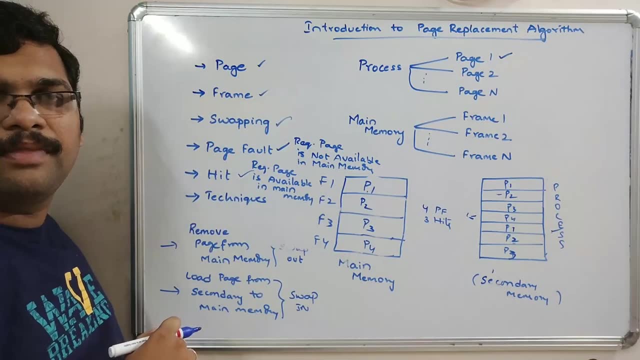 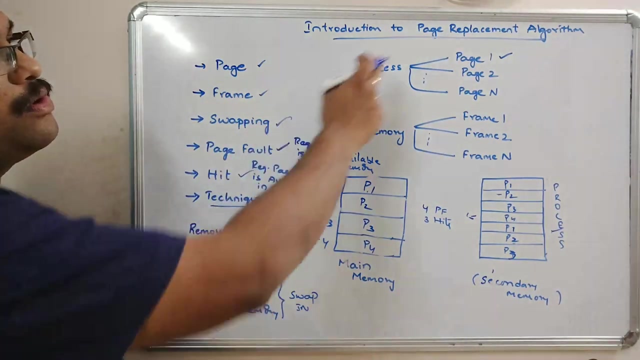 That means the free frames. So if there are no free frames, what we have to do? We have to swap. That means we have to replace one page with the required page So that swapping, that swapping will be taken about these page replacement algorithms. 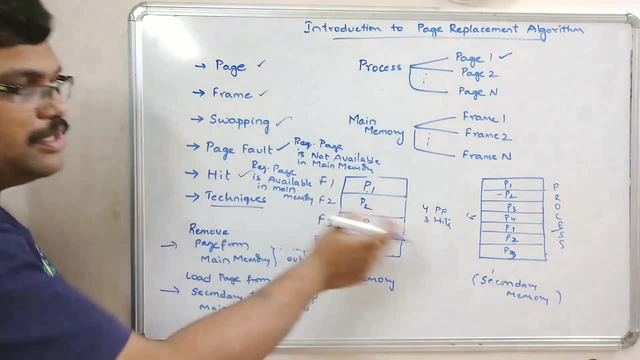 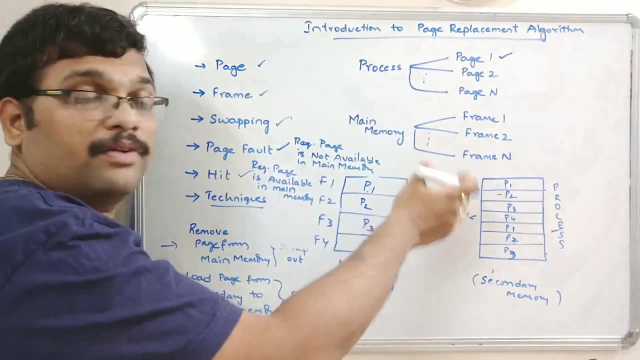 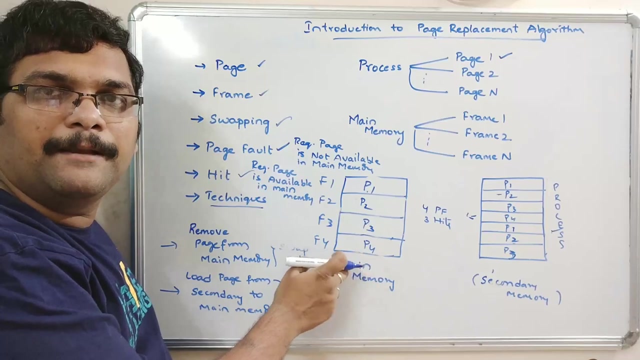 So, based upon the page replacement algorithms, this swapping will be done. So which page have to be replaced from the main memory and which page I mean to replace the required page, So the selection of a page to remove from the main memory. So that is called this page replacement algorithm. 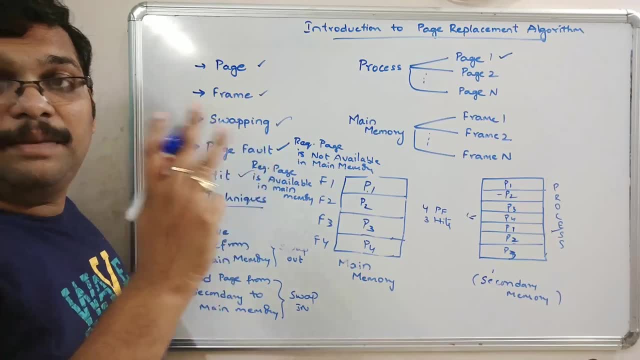 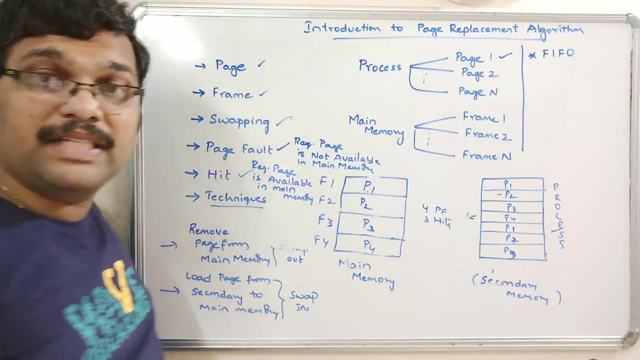 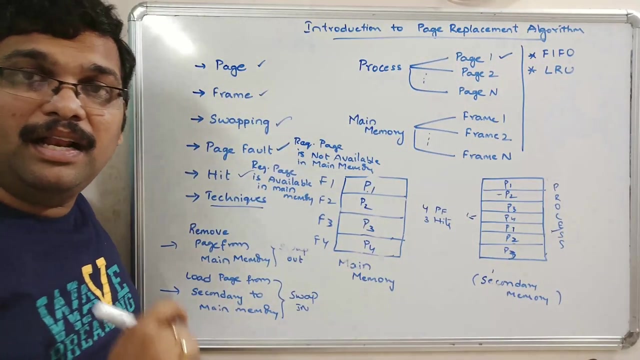 There are three page replacement algorithms. So first one is first in first out, FIFO page replacement algorithm. First in, first out, page replacement LRU, least recently used. page replacement Least recently used. And the third one is optimal page replacement algorithm. Optimal page replacement algorithm. 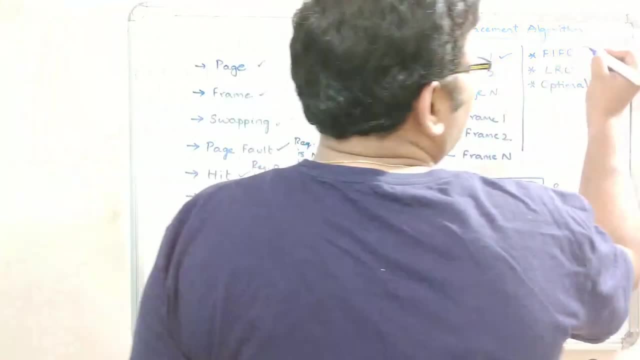 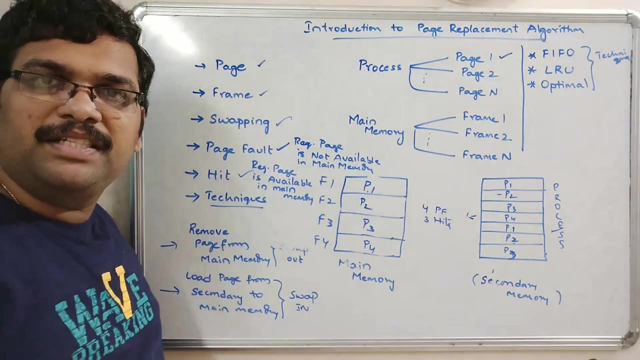 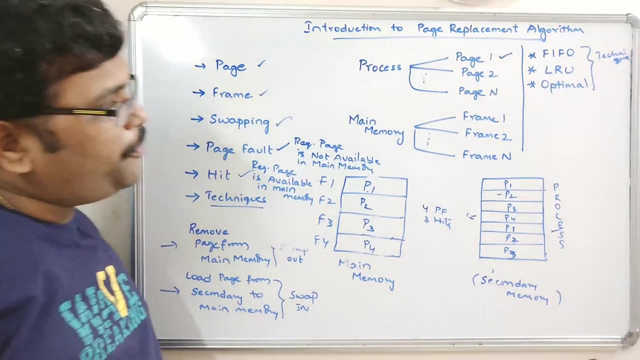 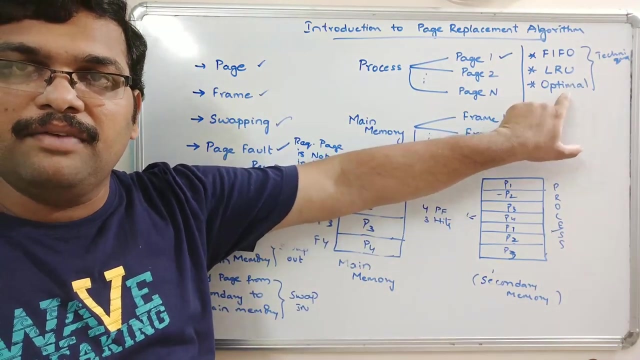 Okay, So these three are nothing but the techniques. techniques to replace the page from the main memory with the secondary memory. that is the required page. okay, so hope you understood this one. So, in order to select which page has to be replaced, depends upon the technique which.